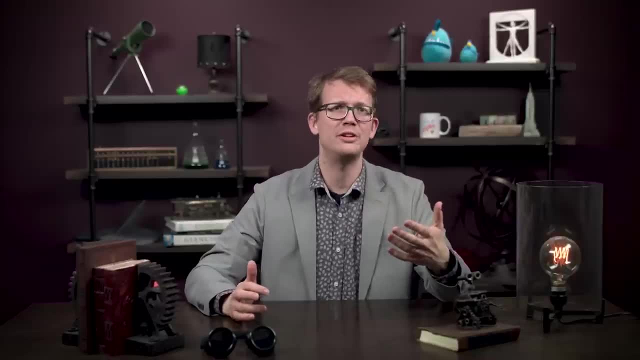 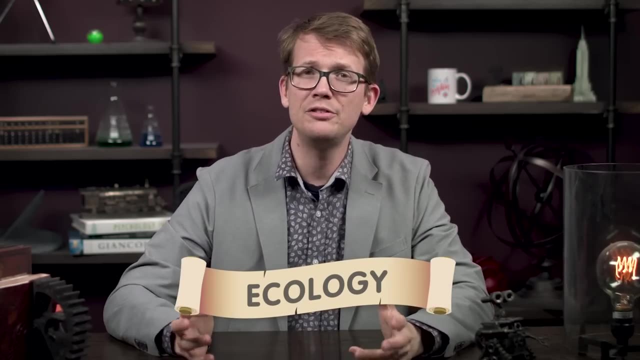 other life science researchers to travel and observe the complexities of the living world And Darwin's German hype man, biologist Ernst Haeckel, coined the word ecology. This means the study of oikos, meaning home or, metaphorically, the environment. 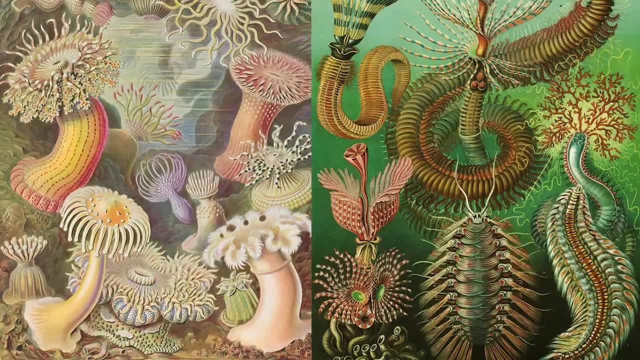 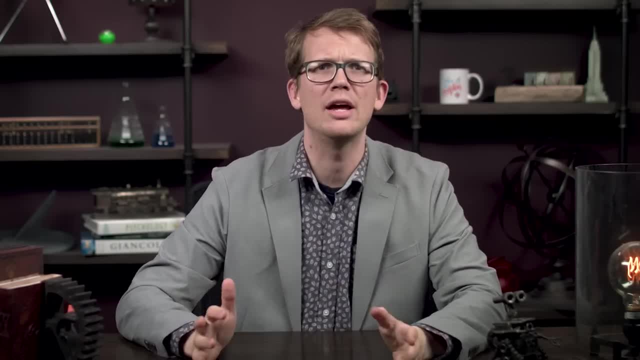 Haeckel introduced popular readers to many environments in his masterwork of scientific illustration: Art Forms in Nature. But okay, what exactly would doing a science of the environment look like? It would involve studying life and the non-living things that affect life, like water and soil. 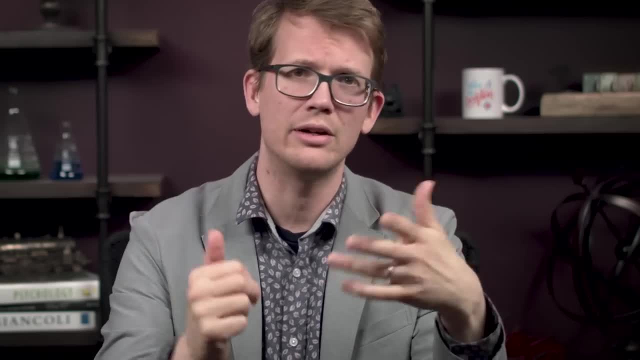 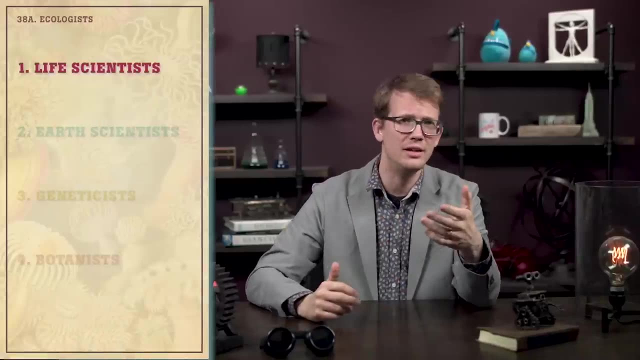 Mediating between the living and non-living things are nutrients like carbon, nitrogen and oxygen, which cycle in and out of organisms in different ways, So early ecologists tend to include life scientists like Haeckel and earth scientists as well. 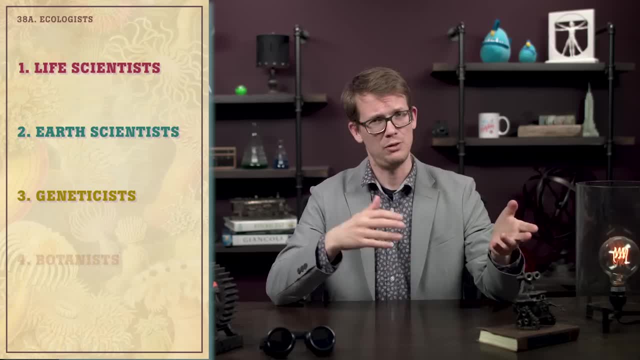 as life scientists like Haeckel, So early ecologists tend to include life scientists like Haeckel and earth scientists, as well as those studying evolution, like geneticists working on flies, and those studying landscapes, like botanists. 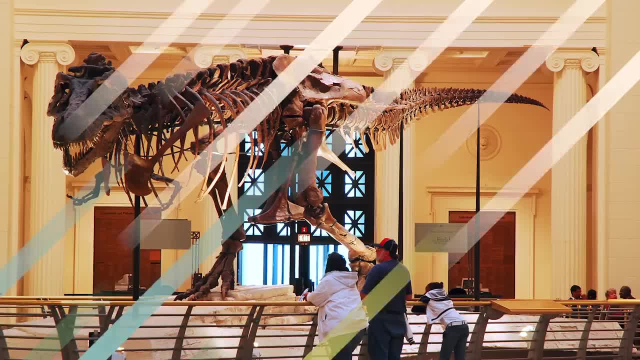 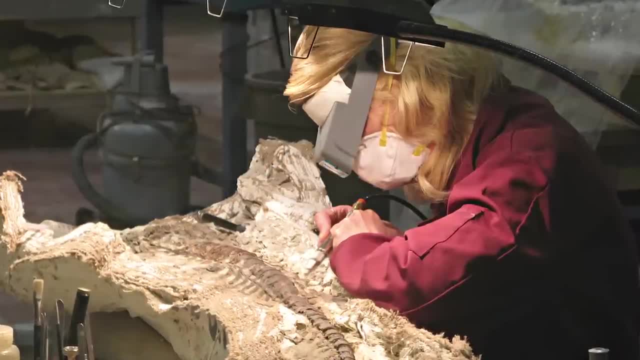 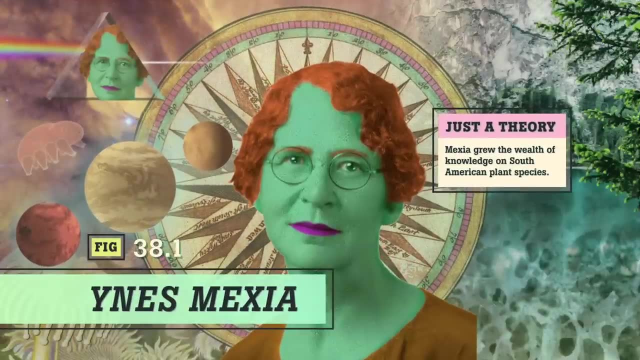 Botanical gardens remained key places to conduct research, as did natural history museums that collected bones, fossils and preserved specimens in jars. Bones could be compared to bones, leaves to leaves, and so on. Mexican-American Inez Mexia started fieldwork at the age of 51, and went on to collect more. 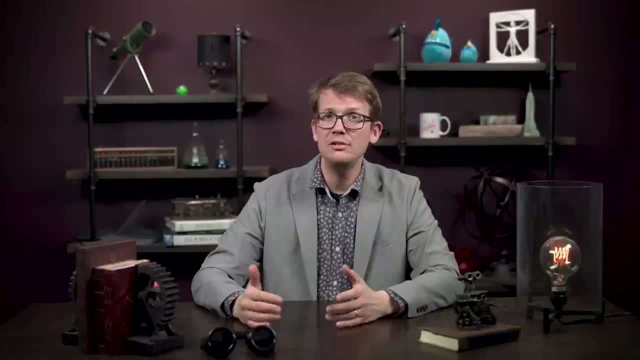 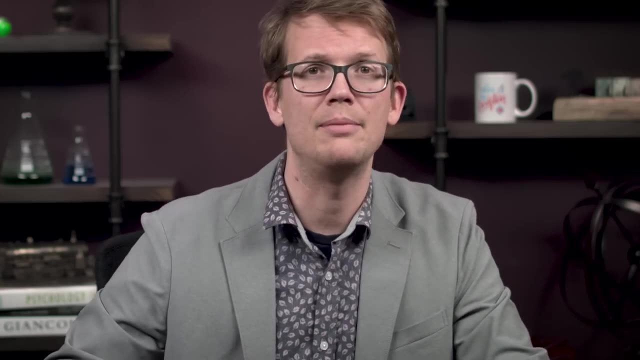 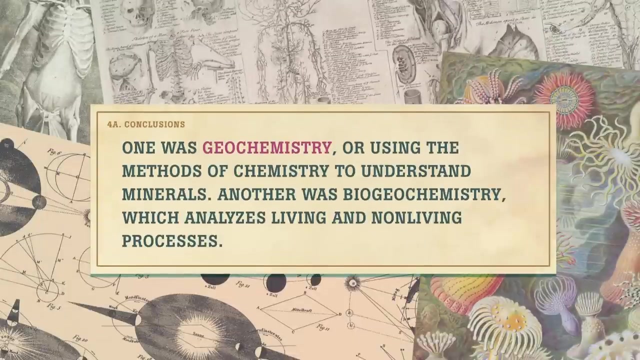 than 150,000 wild botanical specimens, at least 500 of which were new species, And her work is still being processed. Meanwhile, Russian-Ukrainian polymath Vladimir Vernadsky pioneered ways to analyze nature holistically. One was geochemistry, or using the methods of chemistry to understand minerals. 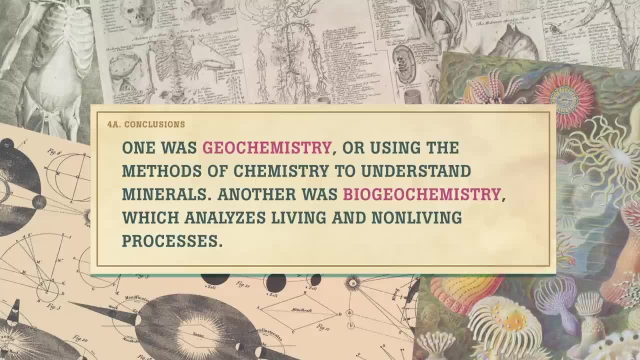 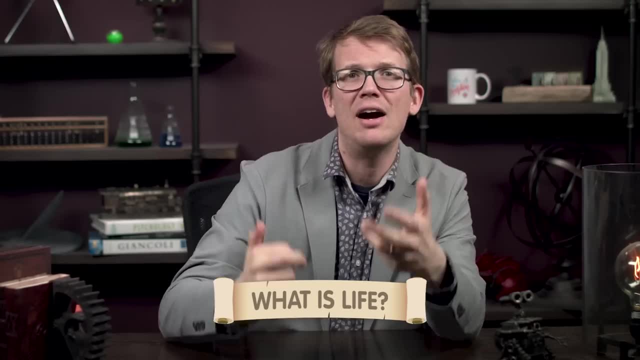 Another was biogeochemistry, which analyzes living and non-living processes. Vernadsky promoted a new mode of ecological thought. What is life? At the highest level of analysis, it's the whole observable-by-humans planet. The non-living, or geochemistry, is the highest level of analysis. 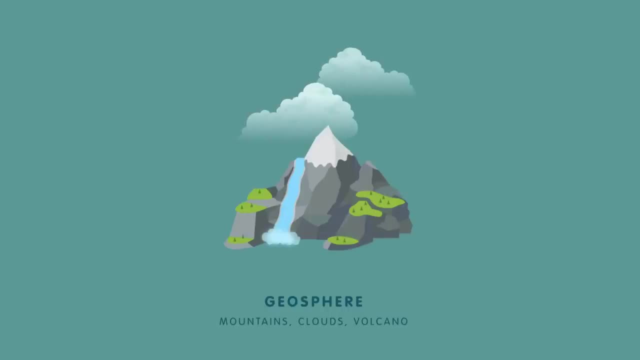 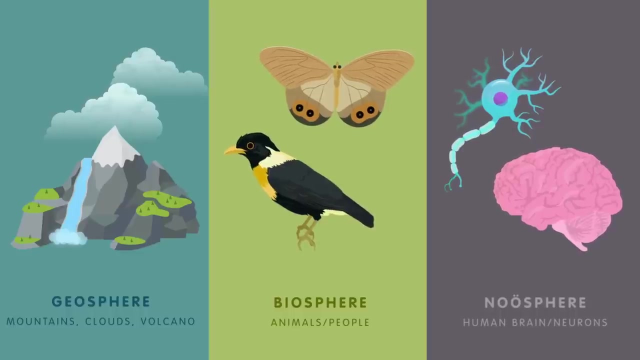 The more abiotic dimension of Earth is the geosphere, which cradles and interacts with the biosphere. Vernadsky even proposed another level, the noosphere, or totality of human thought, which he imagined cradled by and interacting with the lower levels. 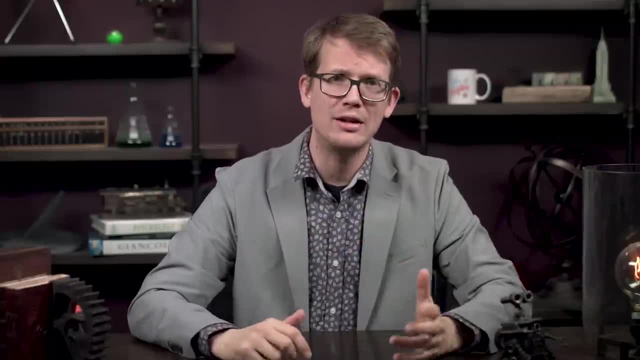 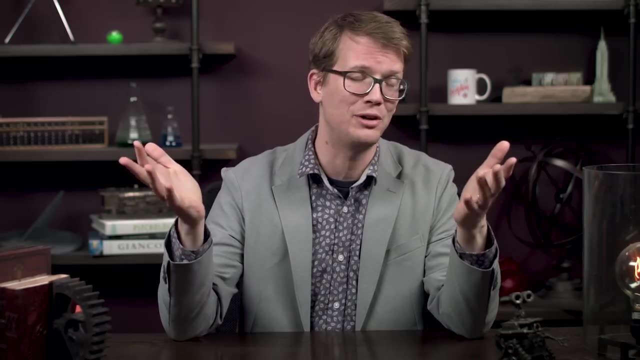 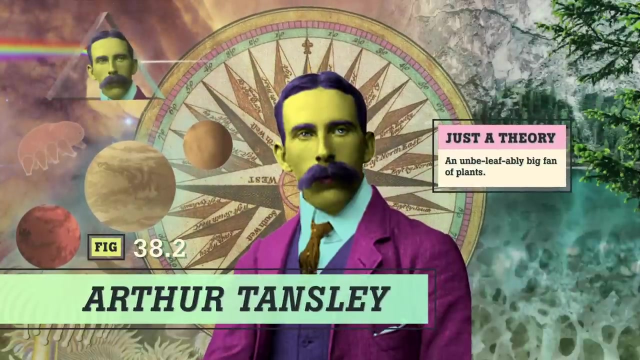 Vernadsky also pioneered radiogeology, the study of radioactive elements in the crust, And he worked on the Soviet's atomic bomb. because so many scientists worked on weapons Around the time that Vernadsky worked, ecology became a discipline. English botanist Arthur Tansley first obsessed over ferns and then later all plants. 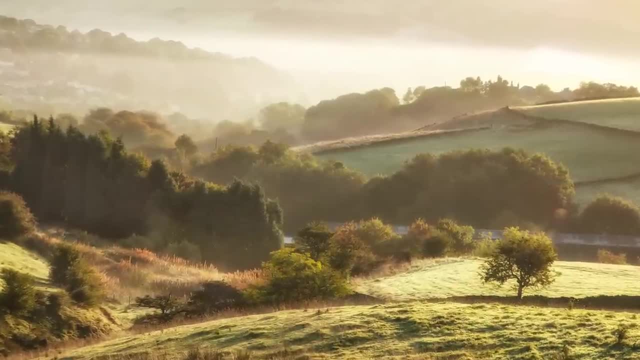 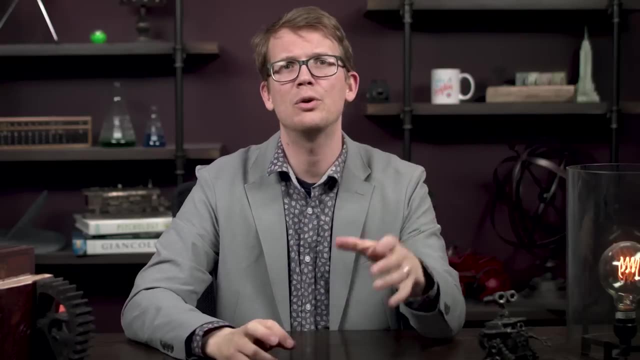 He wanted to map all of the different types of vegetation across England And he thought other botanists should want the same, so he founded clubs to map plant types. In 1913, Tansley organized the first professional society of ecologists and he became the first. 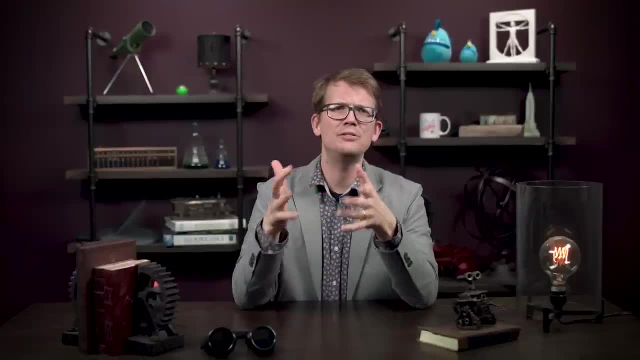 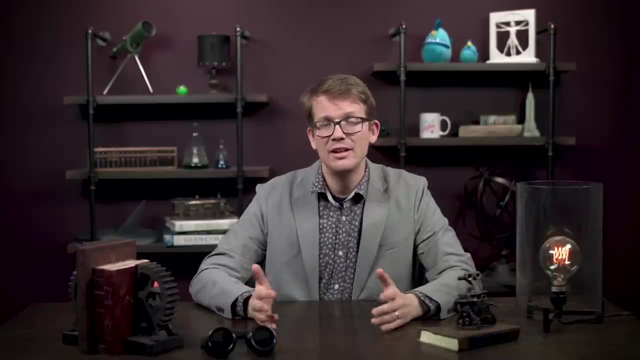 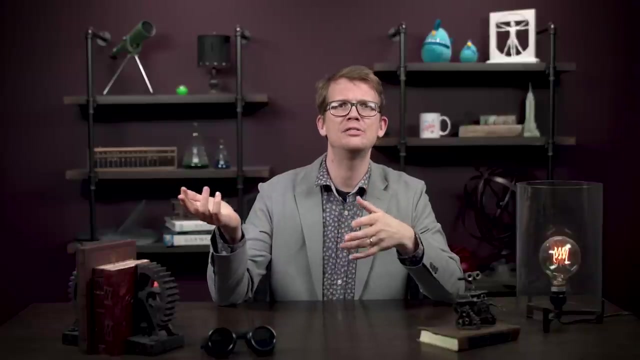 editor of the Journal of Ecology. In terms of epistemic work, Tansley is remembered for one word: Ecosystem. See, scientists are pretty into units. Tansley reframed the study of nature Instead of groups of individual living things. say some birds in some trees, it's the. 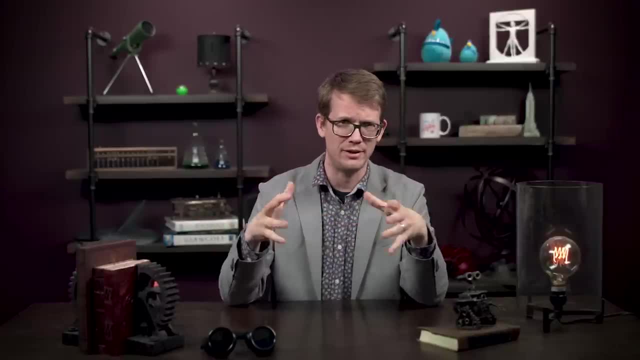 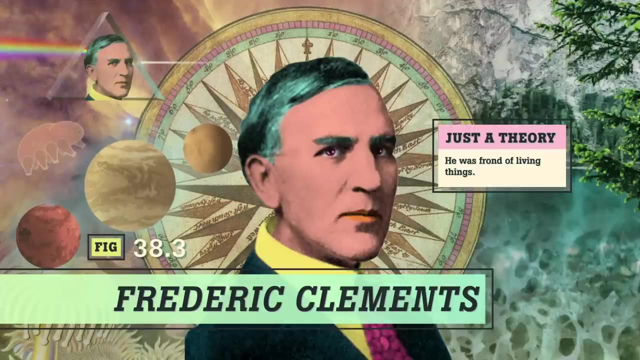 study of dynamic interactions between living and non-living things. in one area, Tansley's rival was American botanist Frederick Clements. His epistemic contributions similarly involved what ecologists should study. Clements argued that plant formations are best studied as units called communities. 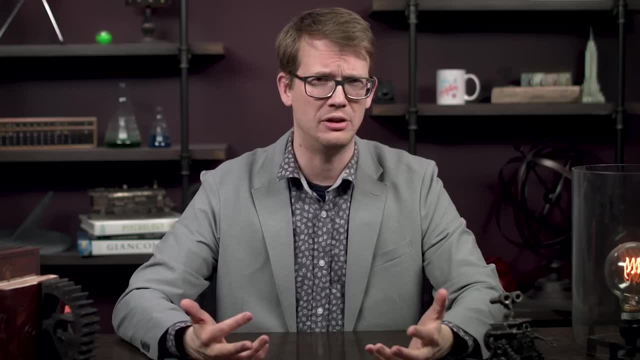 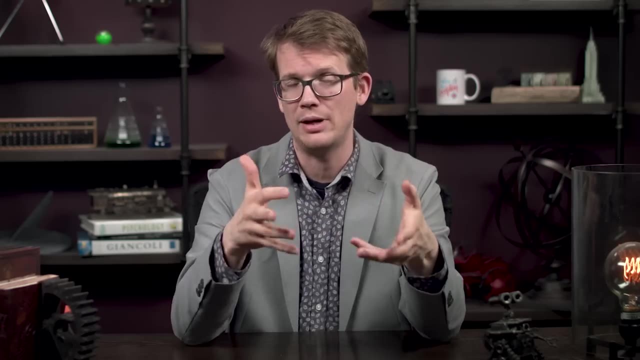 A plant community is not just like a plant, Like a living organism. it is an organism. It's born, grows, eats and dies, And Clements focused on how an area's climate determined which plants will grow there. For example, a pond dries up and becomes first a meadow, then a forest. 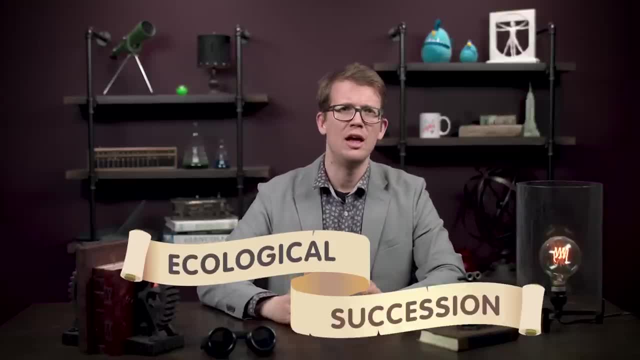 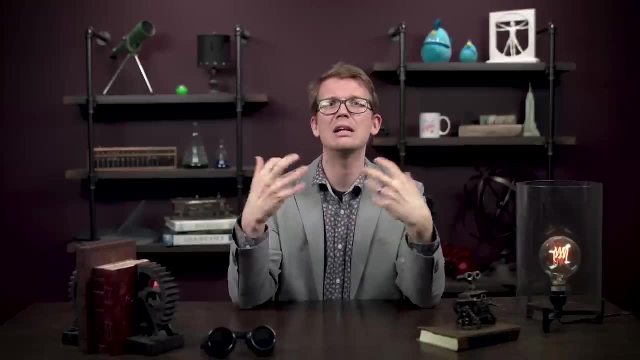 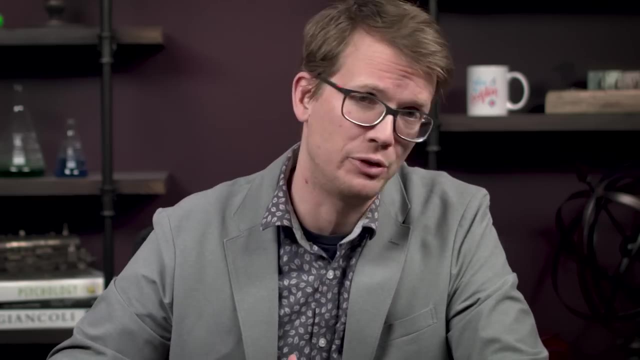 This was a version of an older concept: ecological succession, how the makeup of groups of organisms in areas change over time. But Clements championed his own highly deterministic climax-community version of succession. Tansley hated this. He was arguing that nature is messier than Clements described in his work. 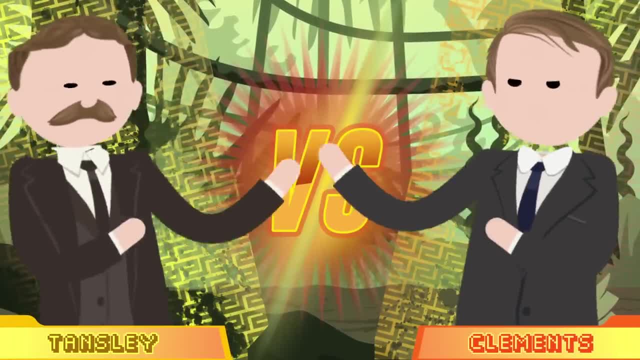 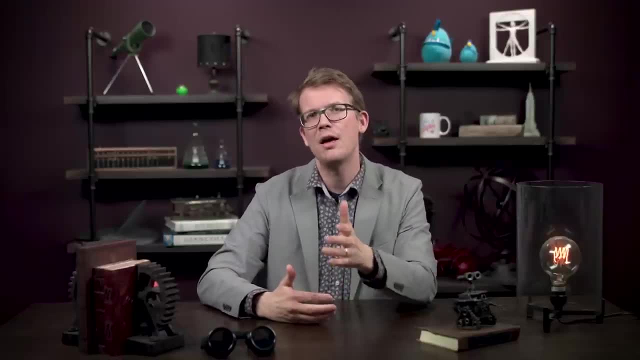 Tansley and Clements fought about ecology from 1905 all the way up to World War II, but both agreed that ecologists should promote conservation or working to actively maintain the health of non-human environments. Conservation has its own history, but ecology as a way of making knowledge has always been. 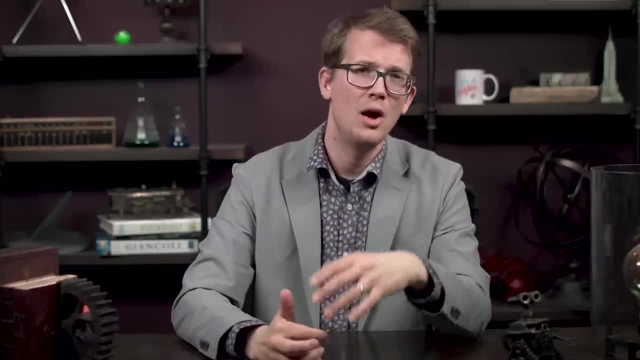 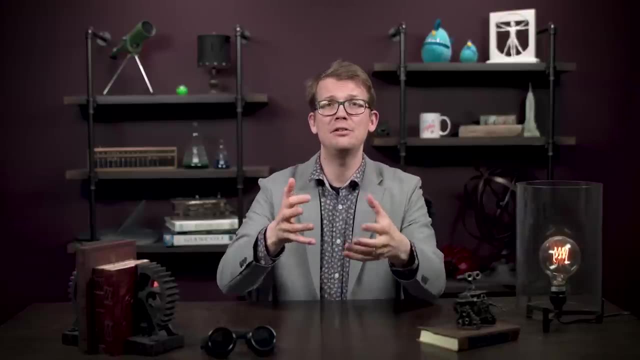 tied to conservation as an ethos or practice, a way of doing something in the world. This isn't a technology, in the same way the light bulb or a computer is, But the practice of conserving ecosystems is as important as lighting up cities or making 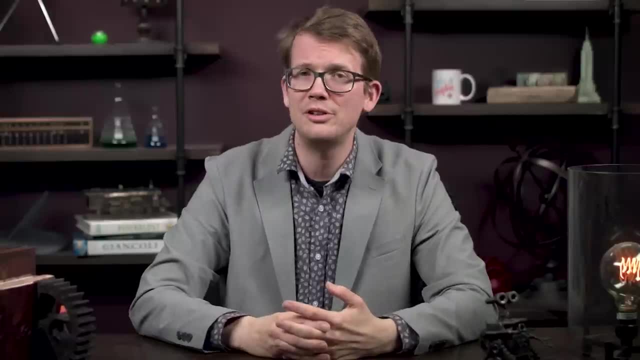 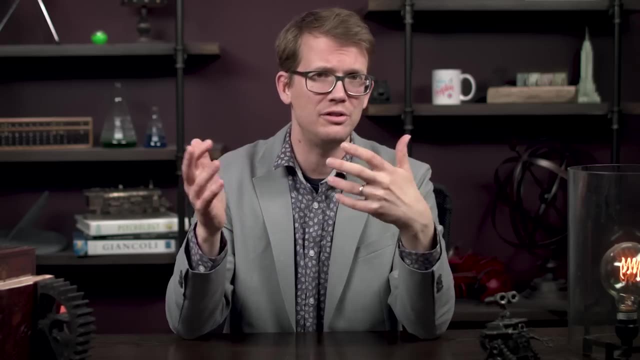 sick memes. To name just two winds in conservation, US President Teddy Roosevelt created the National Park System in the first decade of the 1900s, helping preserve vast areas of forest desert and other wilderness. And in 1972, the Marine Mammal Protection Act helped radically lessen the threat humans 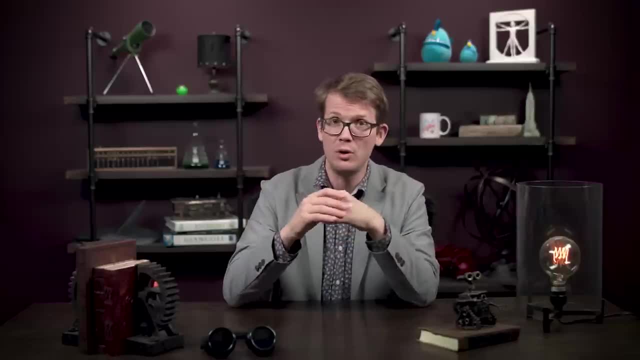 present to dolphins, seals and whales in US waters, Although the threat still remains. But early ecologists didn't have all the tools to do that. They had the tools to do it. They had the tools to do it. They had the tools they needed. 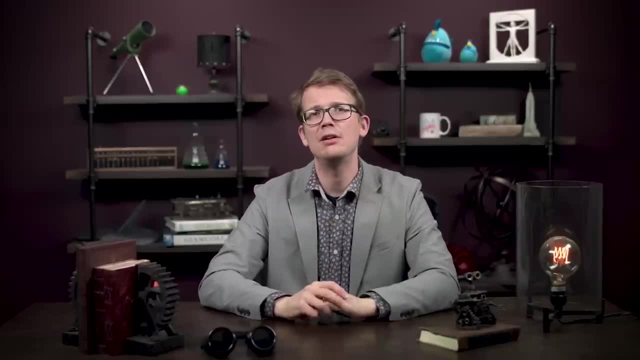 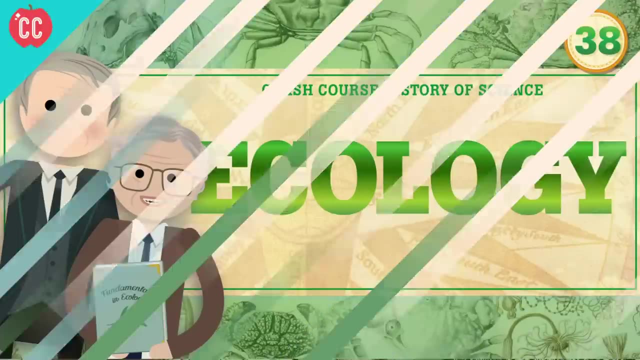 For many of those we can thank English-American polybath George Evelyn Hutchinson, his student Howard T Odom and Howard's older brother Eugene. Take us there Thought Bubble. After World War II they established ecosystem ecology as a richly quantitative discipline. 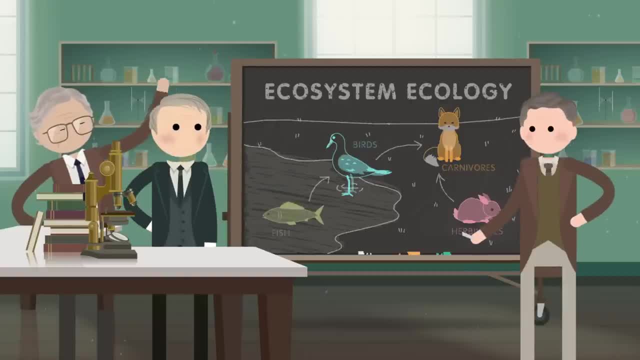 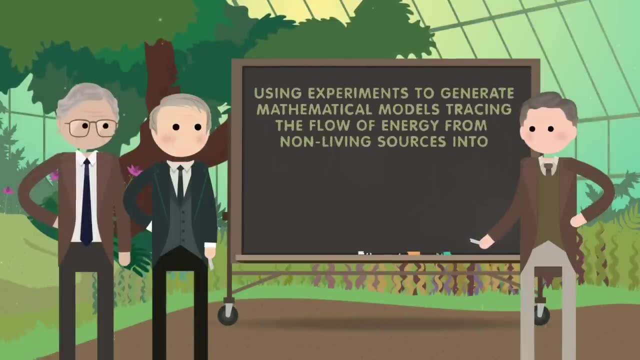 They took Tansley's Essential Insight and ran with it, showing how to model the processes at work in a given ecosystem. All three men used experiments to generate mathematical models tracing the flow of energy. They used the energy from non-living sources into primary producers like plants, primary 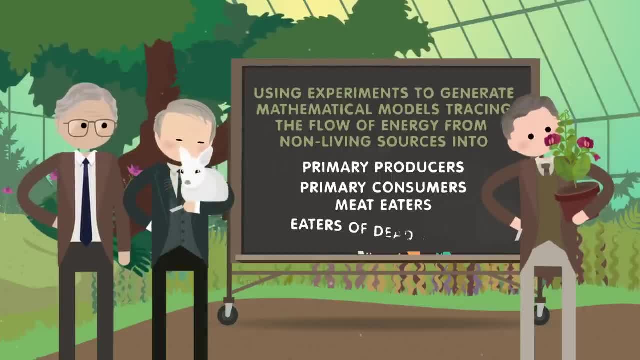 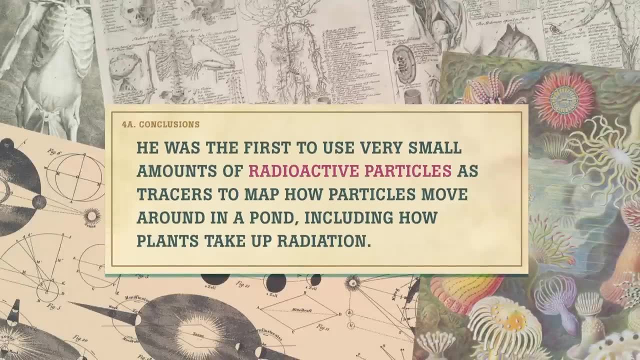 consumers, like herbivores, and then into meat eaters and the eaters of dead things, fungi and bacteria. And he was the first to use very small amounts of radioactive particles as tracers to map how particles move around in a pond, including how plants take up radiation. 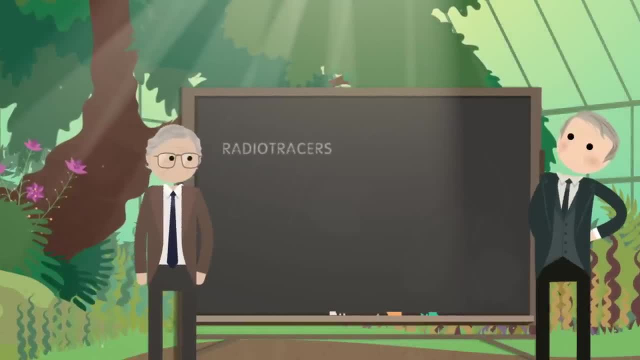 The Odoms went on to develop this radio tracer as tool technique further, which is still used today to study how water moves and how pollutants move through a pond. The Odoms were the first to use this technique to study how water moves and how pollutants. 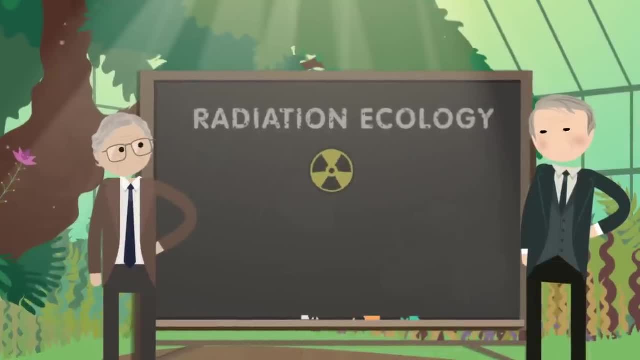 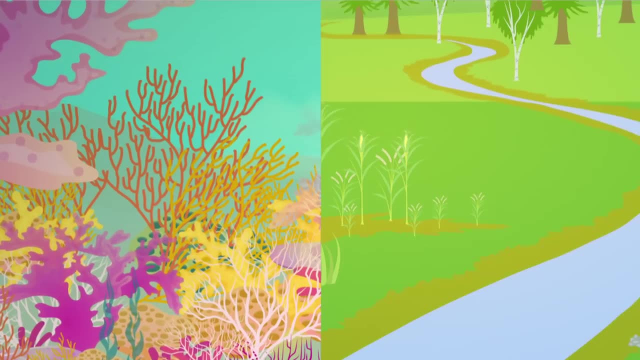 move through a pond. They also helped establish radiation ecology, which studies the effect of radioactive materials on living systems. The Odoms researched ecosystems from coral reefs in the Pacific to riversheds in Georgia. Eugene Odom taught at the University of Georgia actually from 1940 to 2002.. 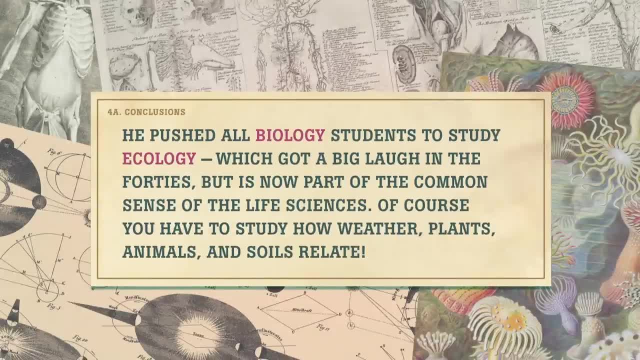 He pushed all biology students to study ecology, which got a big laugh in the 40s but which is now part of the common sense of the life sciences. Of course you have to study how weather, plants, animals and soils relate. 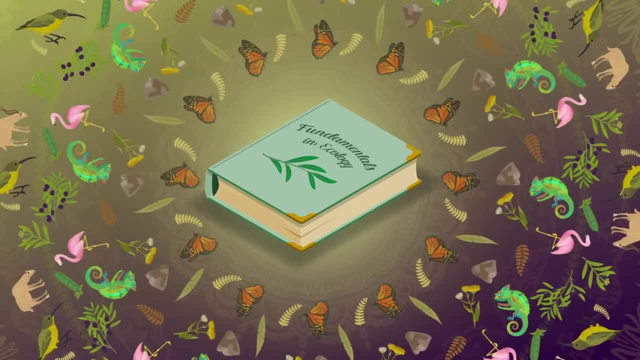 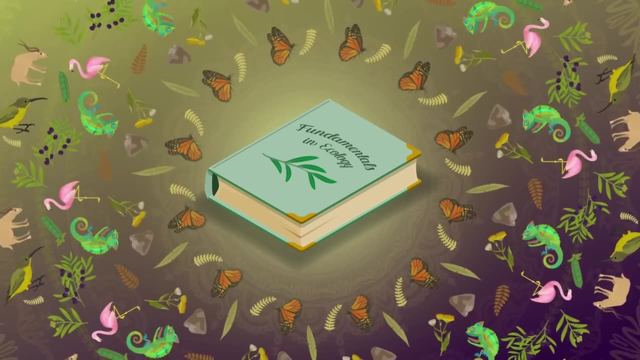 And Eugene deftly summarized with some helpful information. He summarized, with some help from his bro, much of their work in the book Fundamentals in Ecology in 1953. This book unified ecology, offering a range of useful techniques to all budding plant. 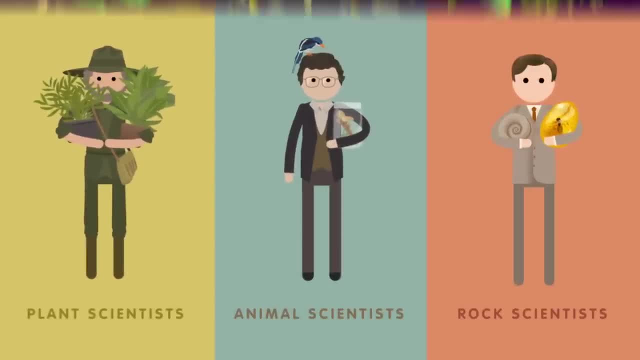 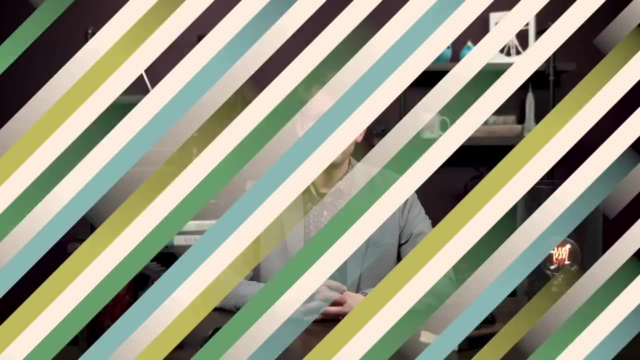 scientists, animal scientists and rock scientists. For years, it was the only textbook in ecology And, revised, it's still used as a textbook in many classes today. Thanks Thought Bubble. The Odoms' work encompassed observational and empirical methods, some of which were 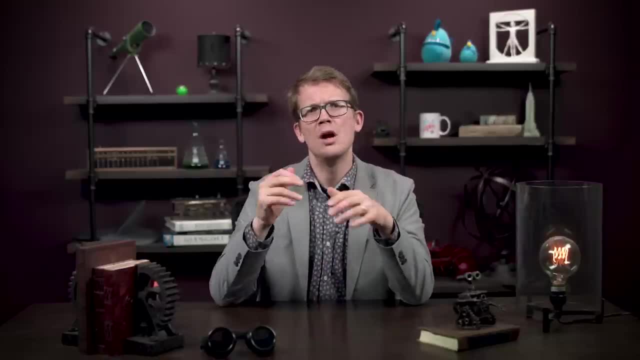 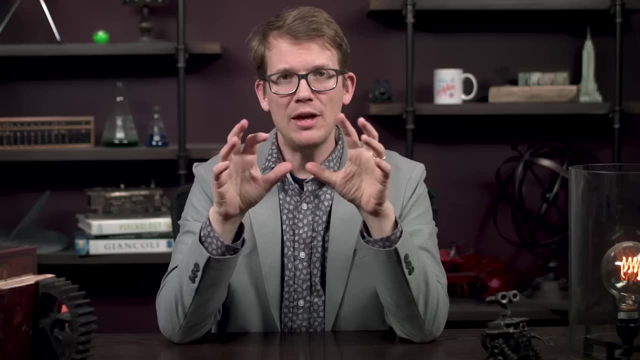 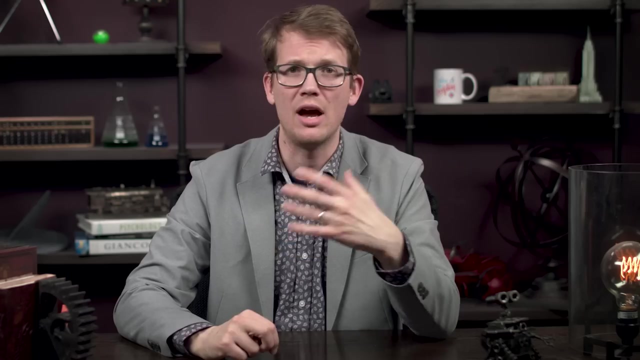 focused on specific parts of ecosystems, But the Odoms were also pioneers of a subdiscipline of ecosystem ecology, confusingly called systems ecology. This is the holistic study of complex living systems as systems, including the interactions among their nonliving inputs, their boundaries, how they adapt to new conditions, how they 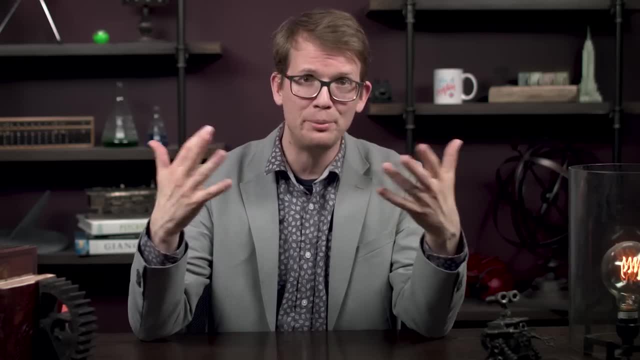 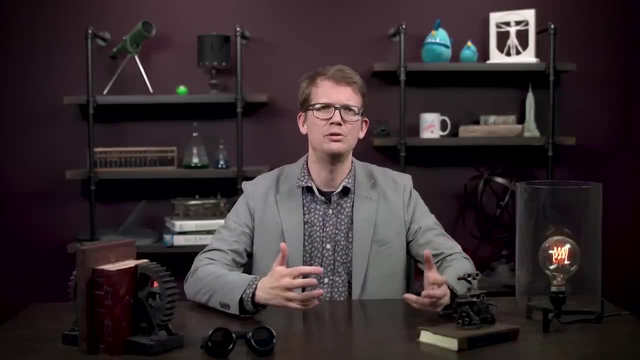 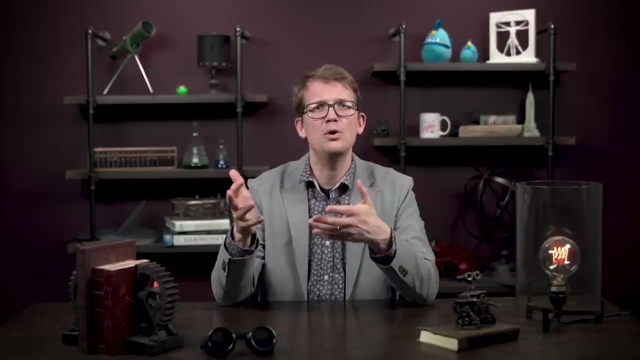 interact with other systems and the unpredictable emergent properties they exhibit. Inspired by Hutchinson's work on feedback loops, Howard modeled how energy flows within ecosystems. He borrowed concepts from thermodynamics and computing in his work on systems ecology. You could even say that the Odoms were trying to understand ecosystems as really complex. 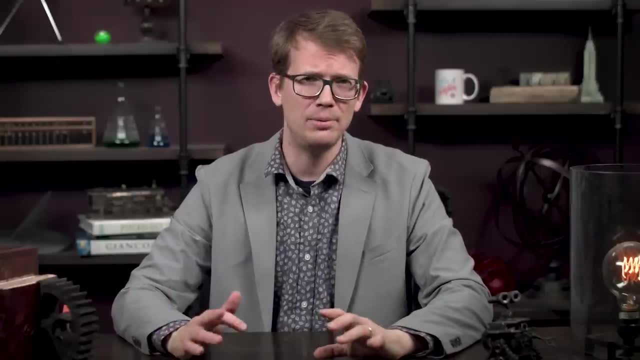 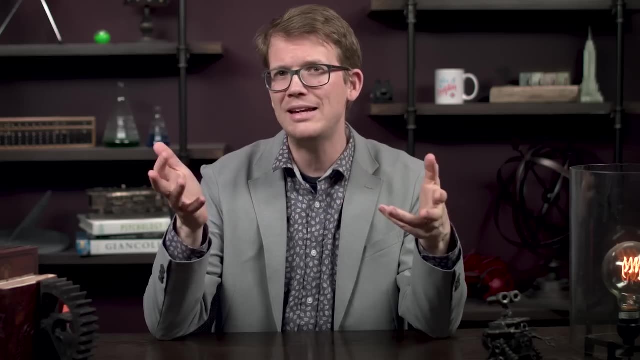 but not random machines. In fact, in the 1960s they applied multiple times for money from NASA to engineer self-regulating closed ecosystems of algae and plankton, a whole biosphere in miniature. These would serve as life-support systems for astronauts. 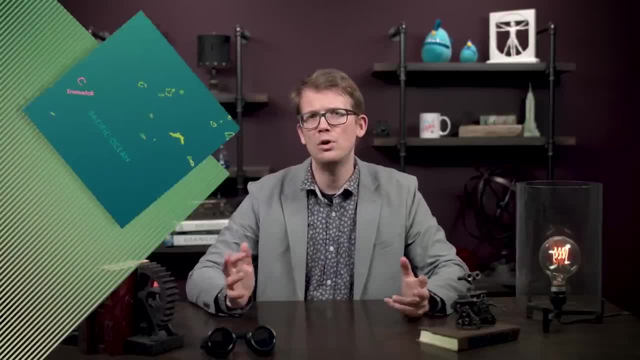 They based their proposals on their study of the energy flows of the ocean. The Odoms, for instance, were trying to understand ecosystems as really complex but not random machines. They were also trying to understand the possibilities of the coral atoll and a wheat hawk in the Marshall. 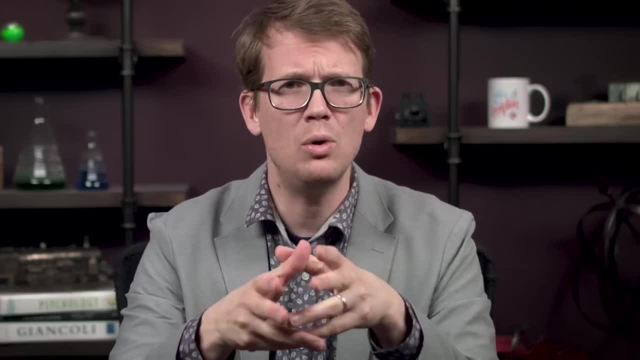 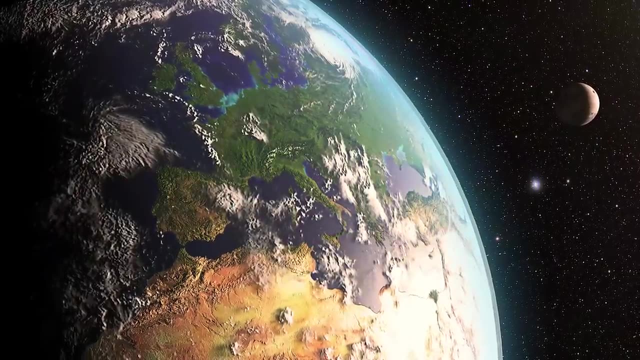 Islands, Alas. NASA thought their plans were too complex and the Odoms returned to earthly matters. The question of life in space intrigued scientists, modeling the relationship between energy, chemicals and organisms. In the 1960s NASA hired English scientist James Lovelock to build instruments to analyze. 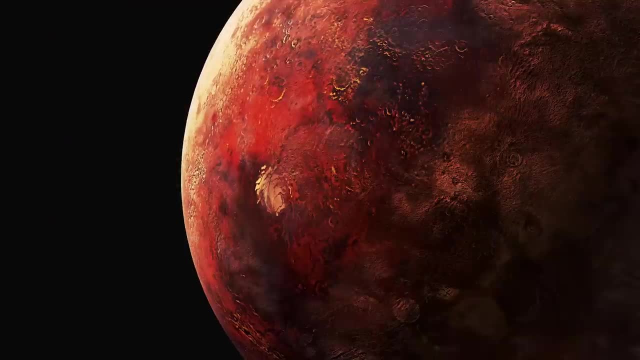 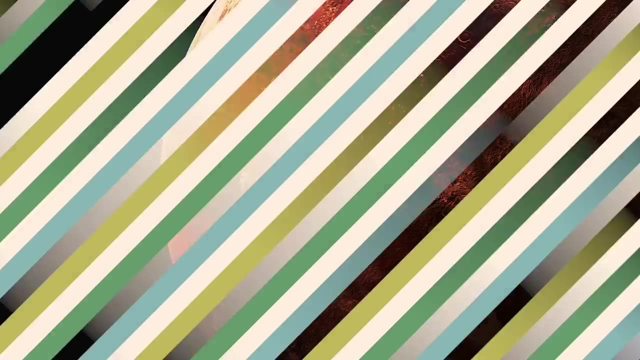 the atmosphere of Mars and look for signs of life. Lovelock thought about why Mars' atmosphere has certain properties different from ours and what that means for the evolution of the ocean, evolution of life. He arrived at the Gaia Hypothesis, named after the Greek Earth Goddess. 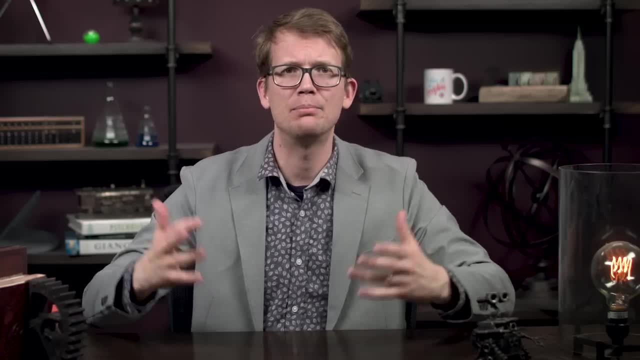 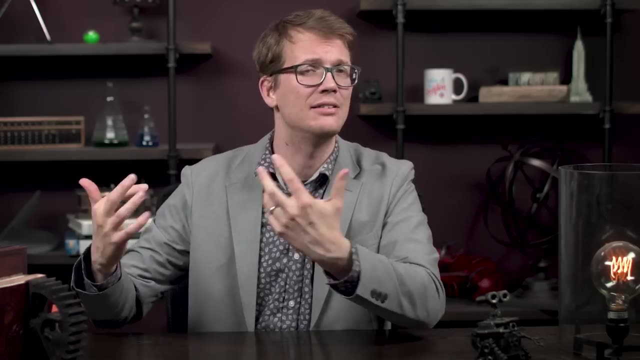 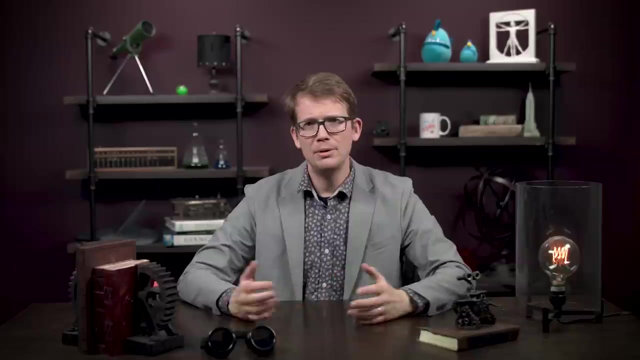 This says the Earth's biogeosphere is self-regulating within broad limits. Living things, air, rocks and water interact in complex ways so that living things can stick around. This was a hugely controversial claim. It suggested a self-awareness to the Earth. 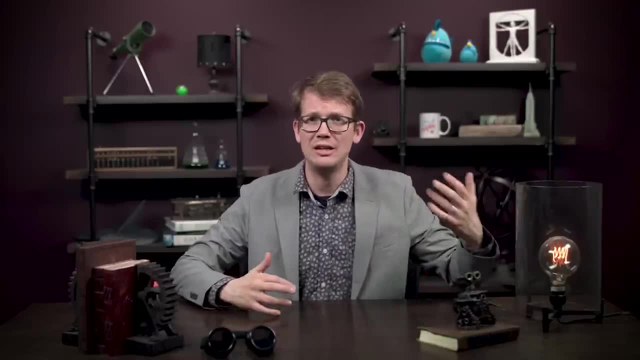 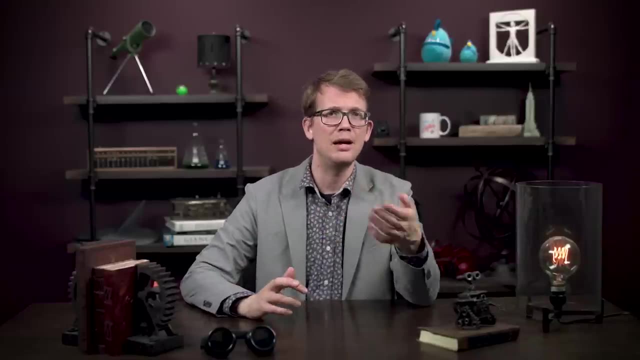 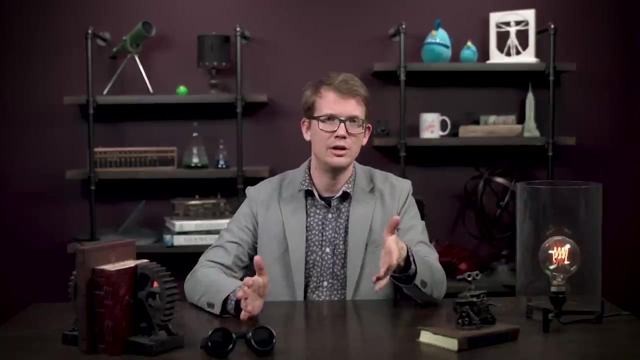 But Lovelock's evidence for a regulatory function between what's in the atmosphere and oceans and what's alive breathing that air or water is pretty convincing And he picked up major support from revolutionary biologist Lynn Margulies. She discovered that some of the tiny organs inside cells, like mitochondria and chloroplasts, 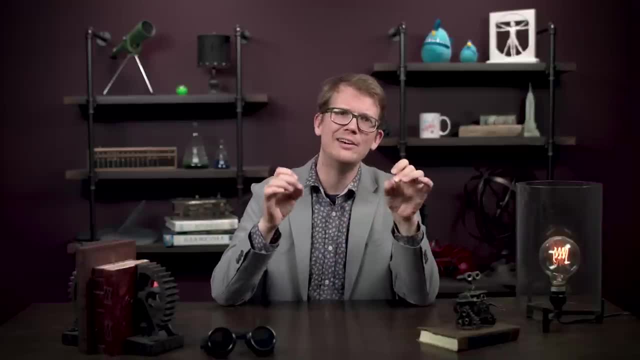 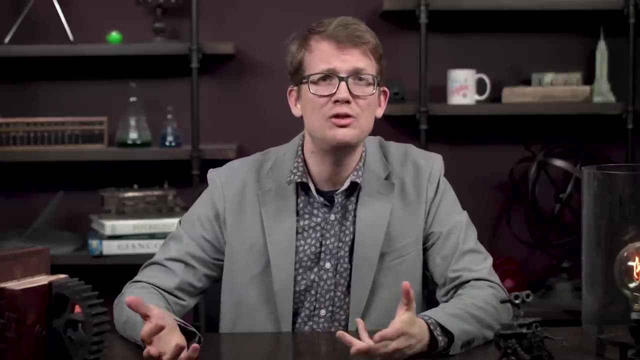 used to be free-floating bacteria that evolved to live entirely within larger organisms. This idea- endosymbiosis- was also hugely controversial, Not because it was too touchy-feely, but because it seemed to have nothing to do with the work of Darwin. 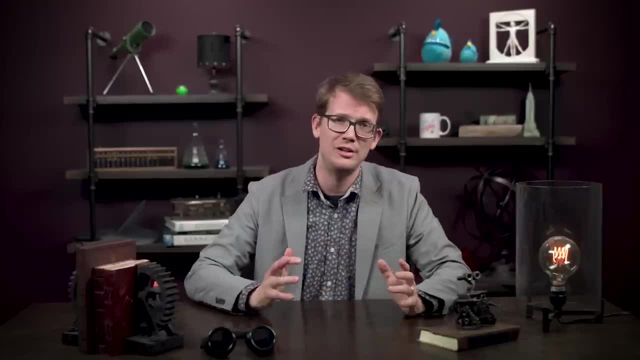 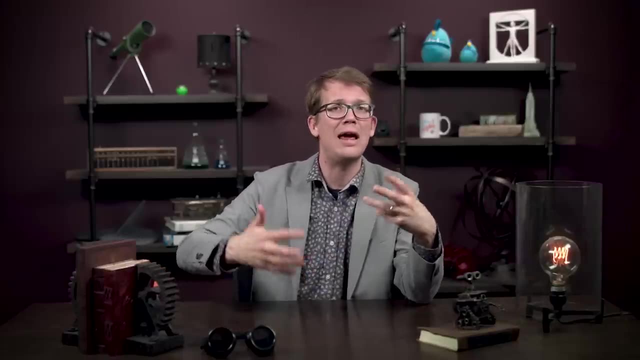 And Margulies also demonstrated lots of evidence. So biologists and ecologists were confronted with complex systems over here, superorganisms over there, communities all the way up and all the way down in scale. Today, this shift is captured in the name of the meta-discipline that applies systems. 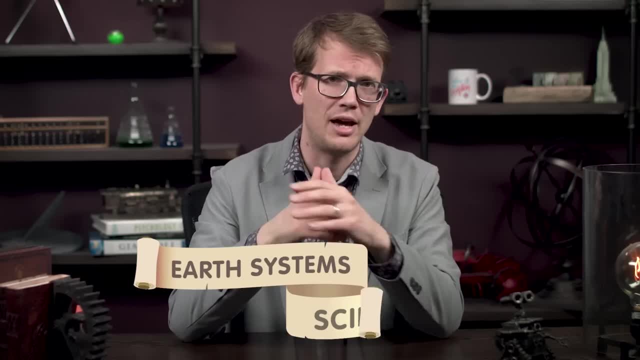 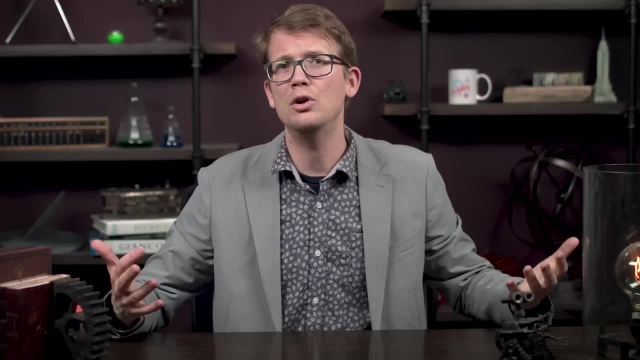 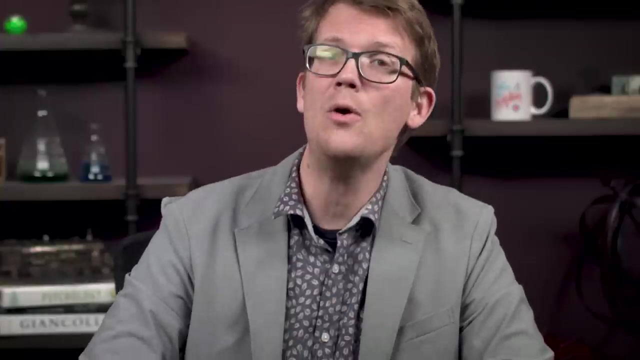 thinking across many sciences: Earth Systems Science. This means understanding how living and non-living processes relate and looking at the entire Earth as one very big but not all universe. But that's not all. There's an infinite house. This is a house we humans can wreck and, we hope, repair. 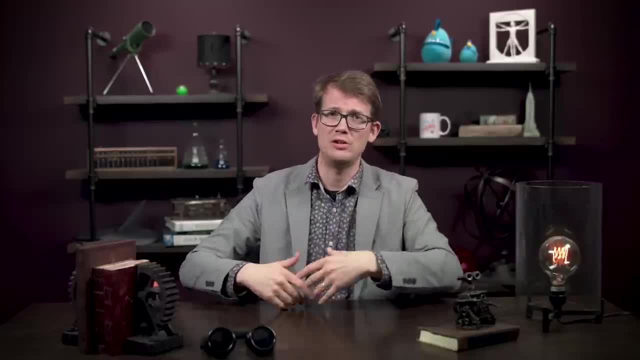 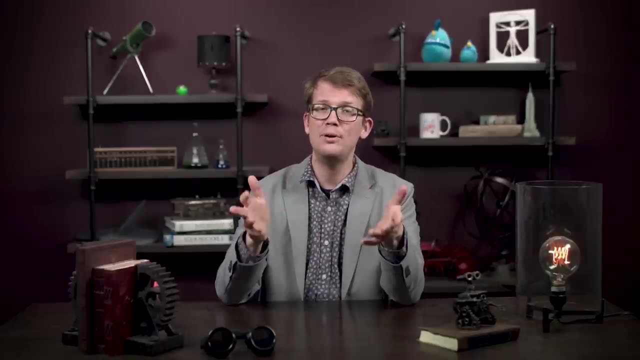 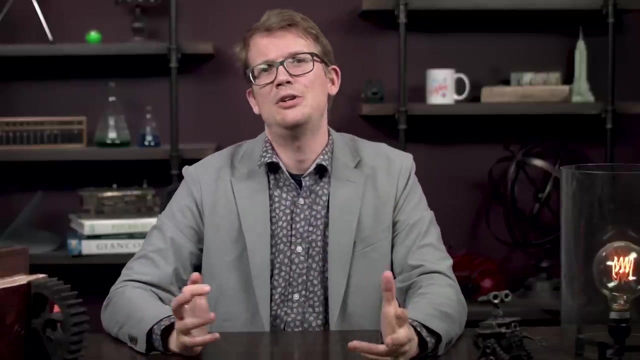 So just as the life sciences had to scale up to ecosystems and then to the entire Earth, they had to take into account how humans affect ecosystems and Earth systems. A new branch human ecology developed. If that all sounds a bit like what Vernadsky said a hundred years ago, you're right. 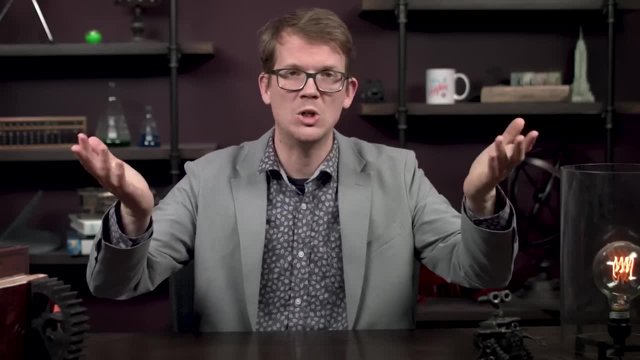 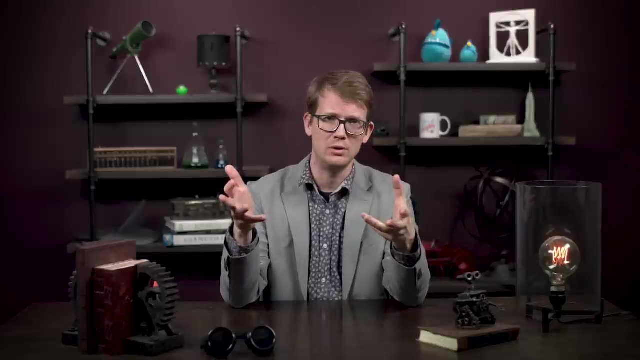 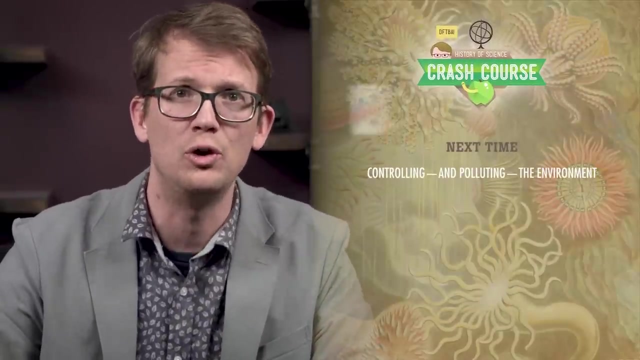 Human thought, non-human life, rocks, water, all connected. Or, as Eugene Odom wrote, The landscape is not just a supply depot, but is also the oikos, the home in which we must live. Next time we'll move from studying nature to controlling it and losing control. 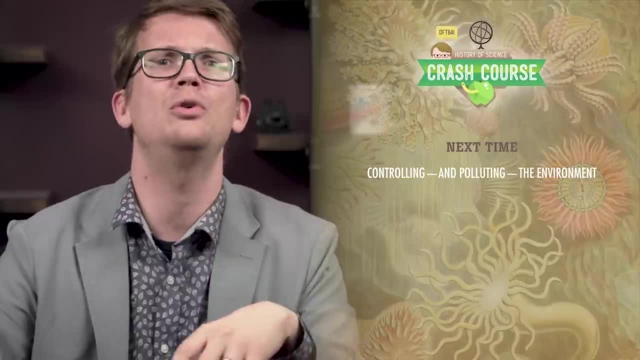 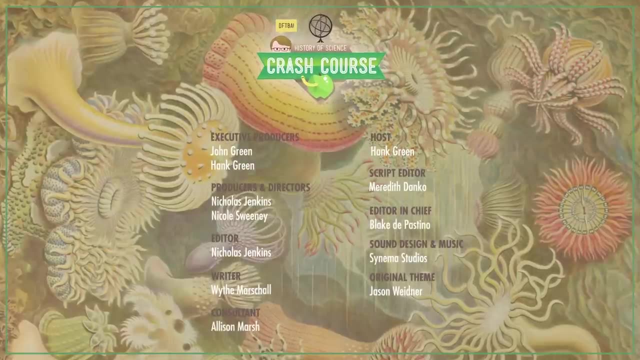 It's time for the Green Revolution, pesticide pollution and the birth of environmentalism. Crash Course History of Science is filmed in the Dr Cheryl C Kinney Studio in Missoula, Montana, and it's made with the help of all these nice people and our animation team. 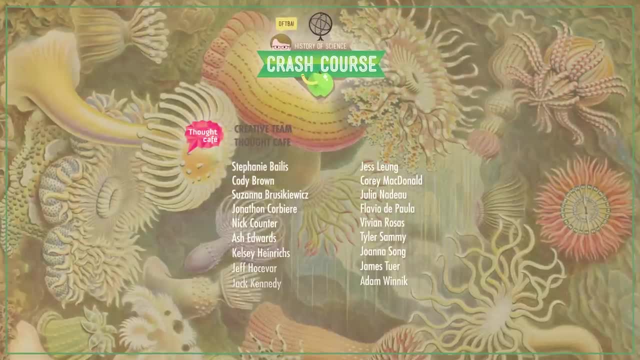 is Thought Cafe Crash Course is a Complexly production. If you want to keep imagining the world complexly, you can watch it here. Thanks for watching. You can check out some of our other channels, like The Art Assignment, Nature League and. 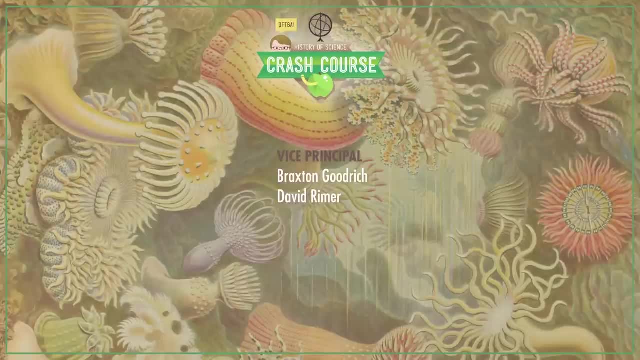 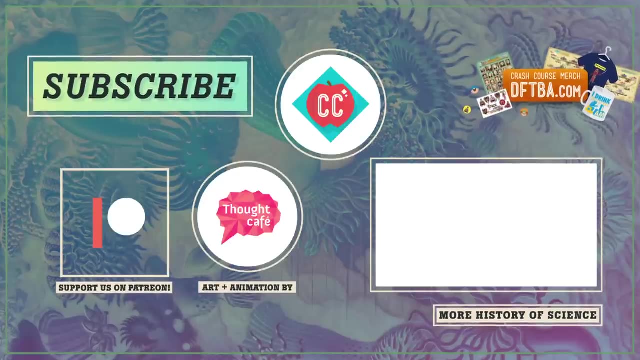 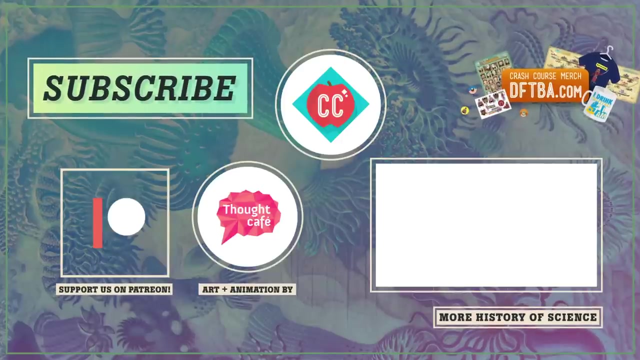 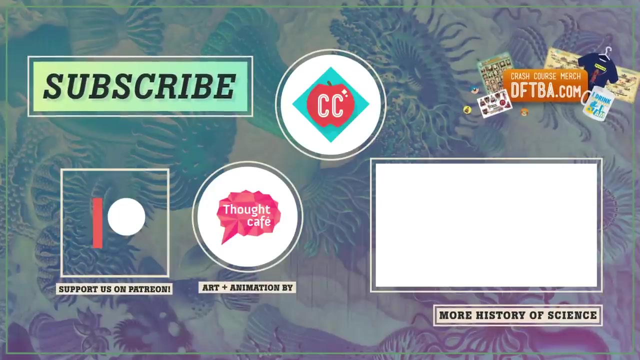 Sideshow Space. We'll see you next time.